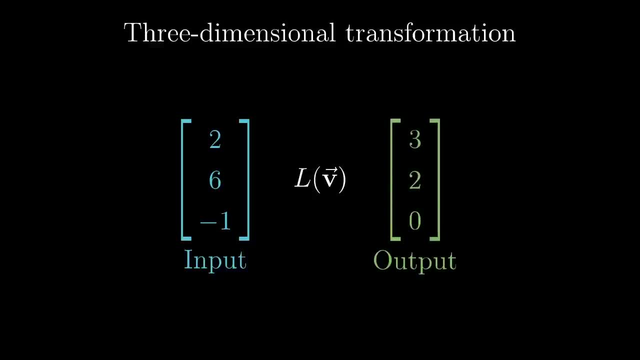 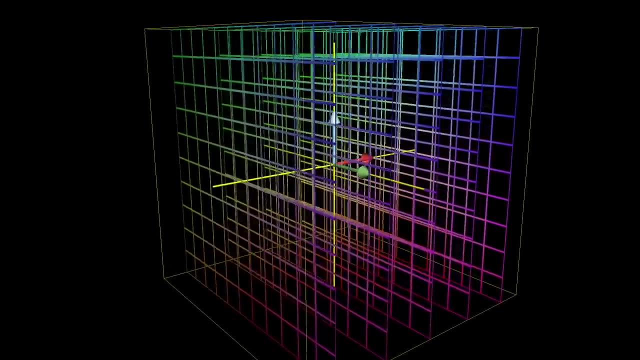 vectors as inputs and three-dimensional vectors as outputs. We can visualize this by smooshing around all the points in three-dimensional space, as represented by a grid, in such a way that keeps the grid lines parallel and evenly spaced and which fixes the origin. 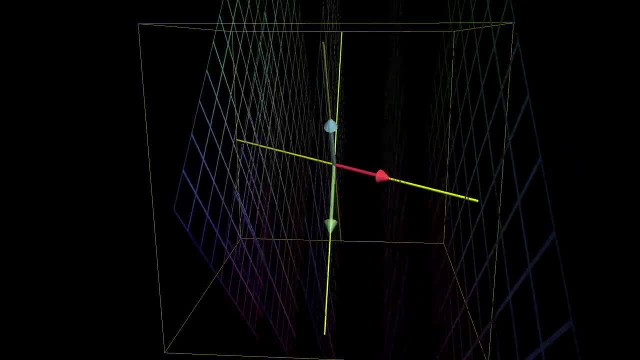 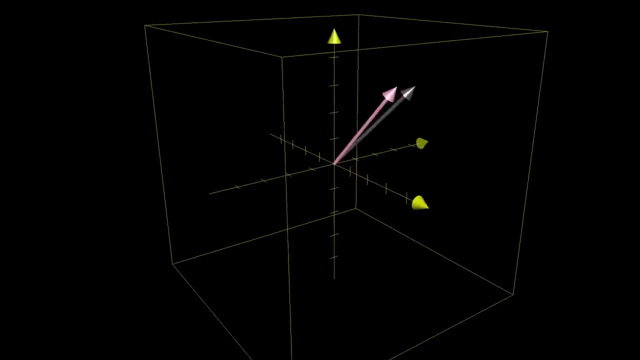 in place And, just as with two dimensions, every point of space that we see moving around is really just a proxy for a vector who has its tip at that point, and what we're really doing is thinking about input vectors moving over two dimensions. 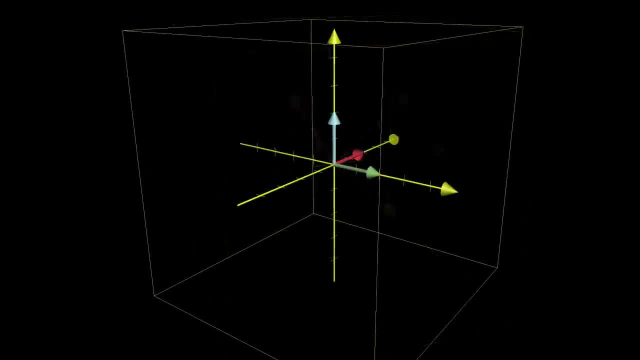 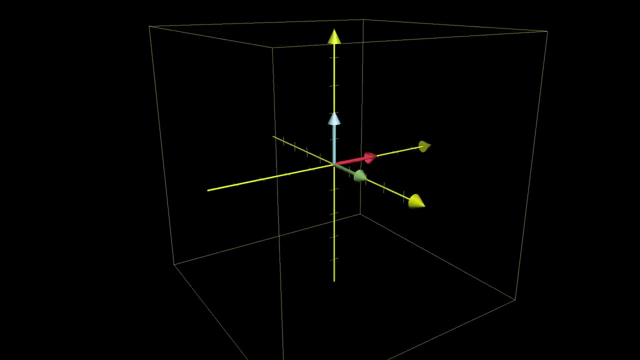 And, just as with two dimensions, one of these transformations is completely described by where the basis vectors go. But now there are three standard basis vectors that we typically use: The unit vector in the x-direction, i-hat. the unit vector in the y-direction, j-hat. 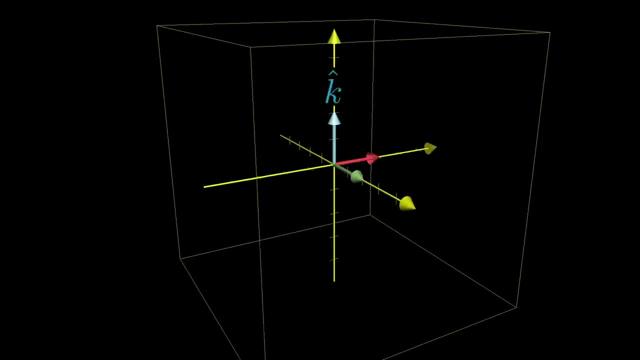 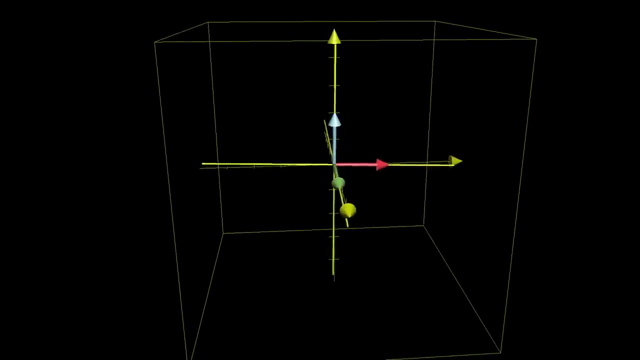 and a new guy, the unit vector in the z-direction called k-hat. In fact, I think it's easier to think about these transformations by only following those basis vectors, since the full 3D grid representing all points can get kinda messy. 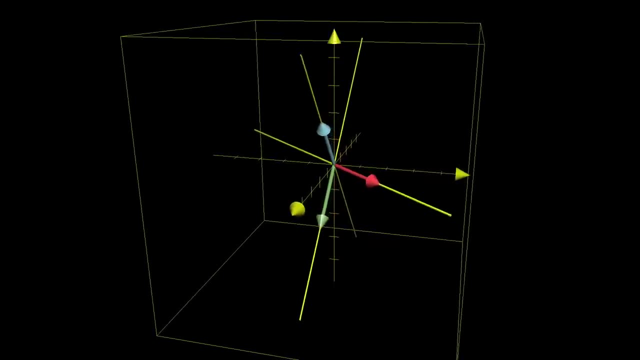 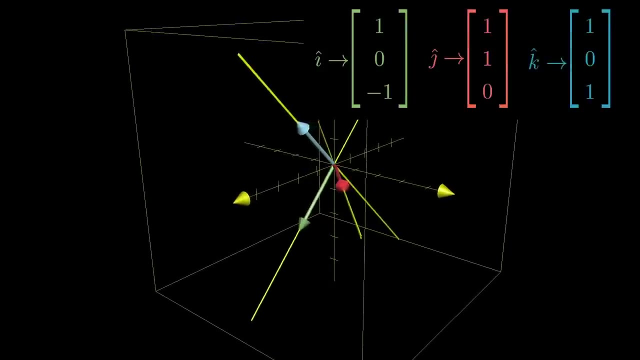 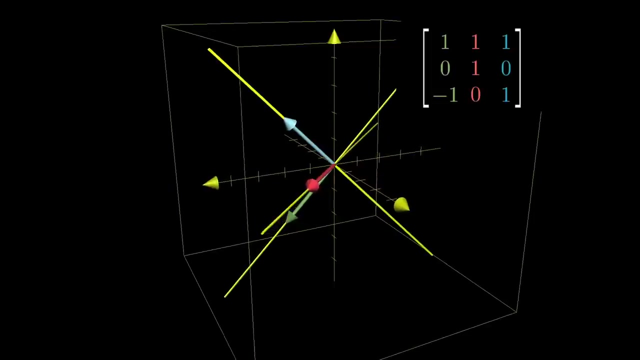 By leaving a copy of the original axes in the background, we can think about the coordinates of where each of these three basis vectors lands. Record the coordinates of these three vectors as the columns of a 3x3 matrix. This gives a matrix that completely describes the 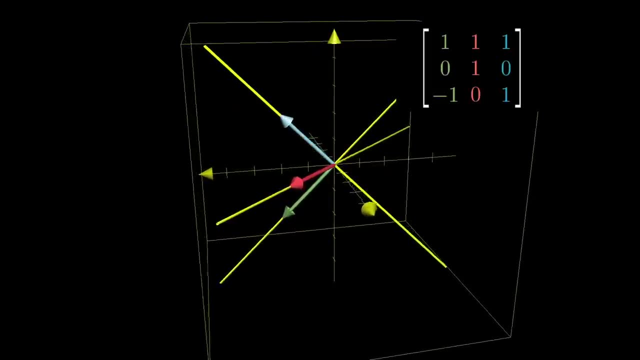 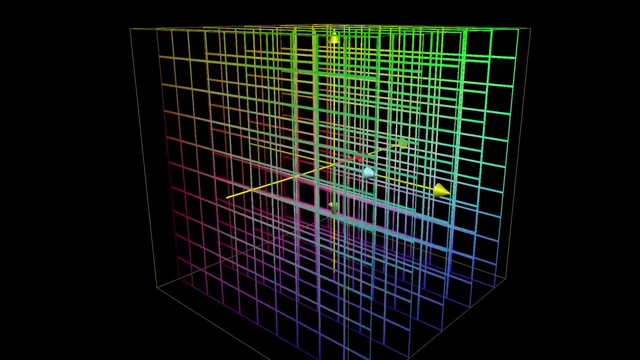 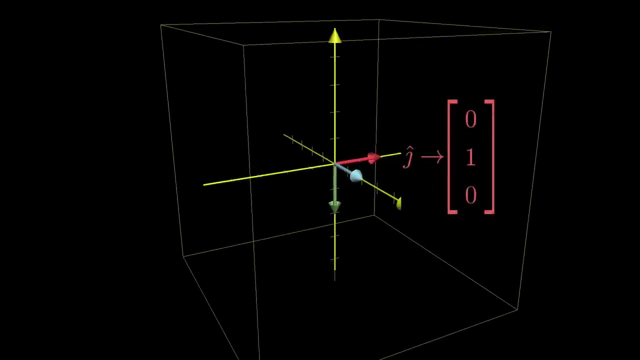 transformation using only nine numbers. As a simple example, consider the transformation that rotates space 90 degrees around the y-axis. So that would mean that it takes i-hat to the coordinates on the z-axis. it doesn't move j-hat, so it stays at the coordinates. 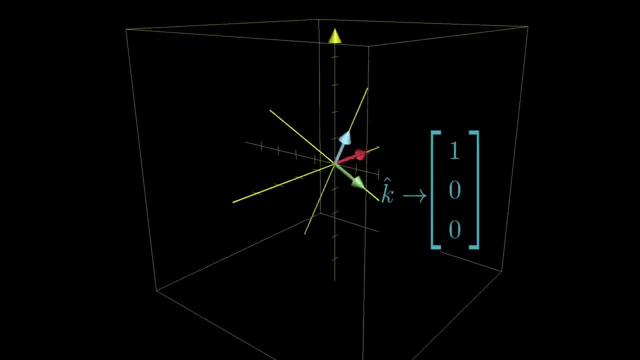 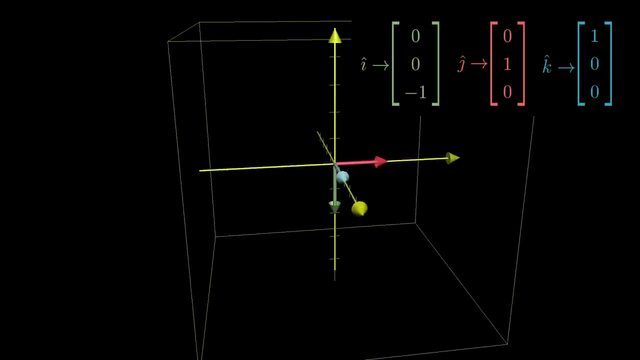 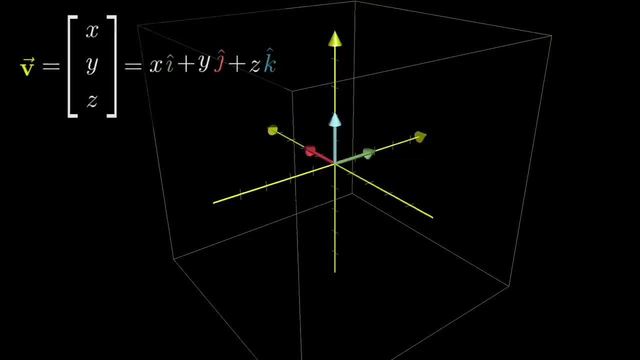 and then k-hat moves over to the x-axis at, Those three sets of coordinates become the columns of a matrix that describes that rotation transformation To see where a vector with coordinates lands. the reasoning is almost identical to what a 2D matrix does. Each of those coordinates can be thought of as instructions for how. 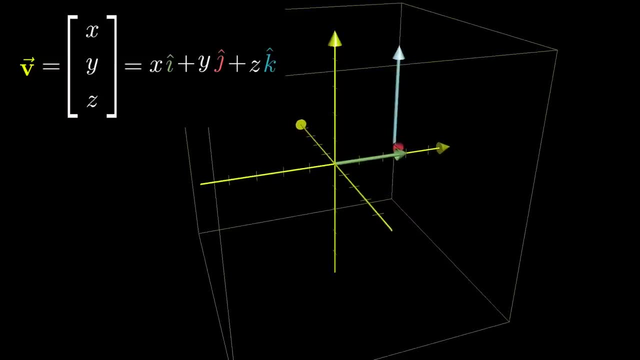 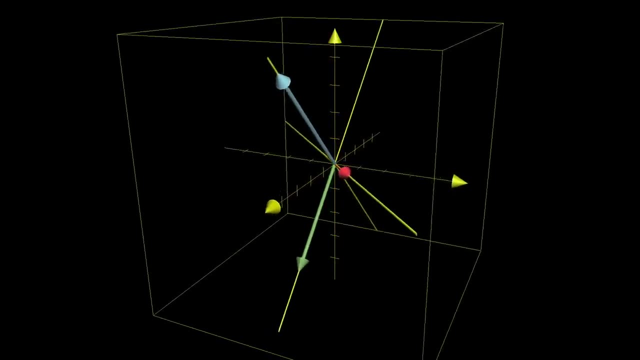 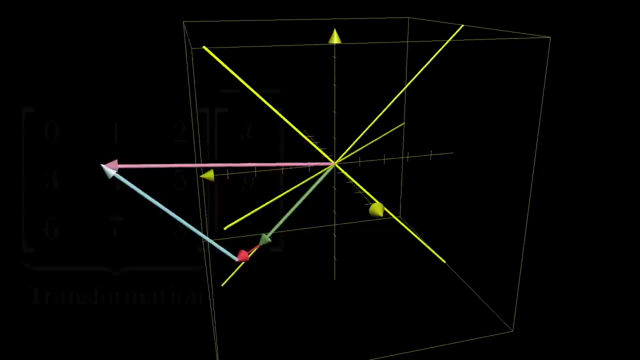 to scale each basis vector so that they add together to get your vector. And the important part, just like the 2D case, is that this scaling and adding process works both before and after the transformation. So to see where your vector lands, you multiply those coordinates. 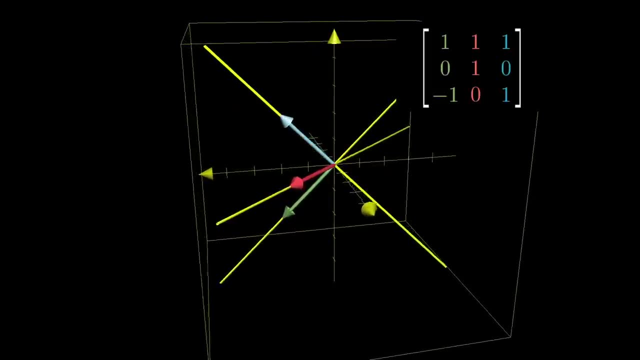 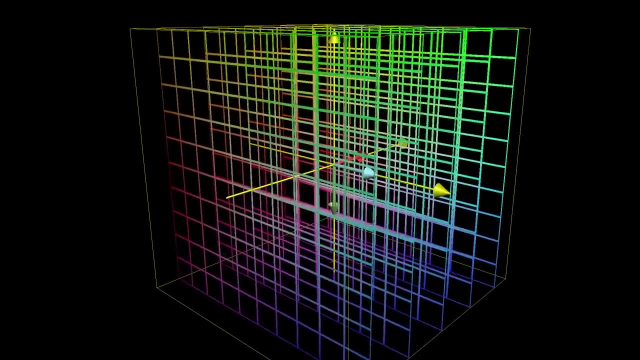 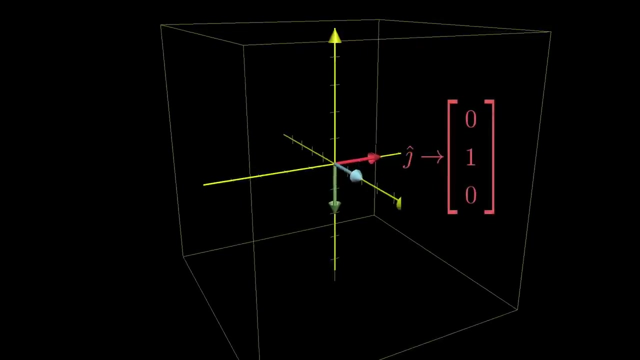 transformation using only nine numbers. As a simple example, consider the transformation that rotates space 90 degrees around the y-axis. So that would mean that it takes i-hat to the coordinates on the z-axis. it doesn't move j-hat, so it stays at the coordinates. 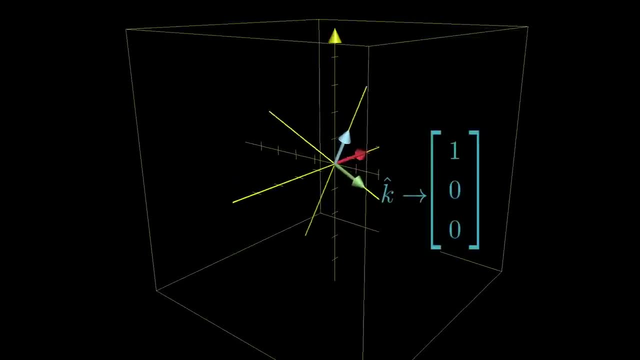 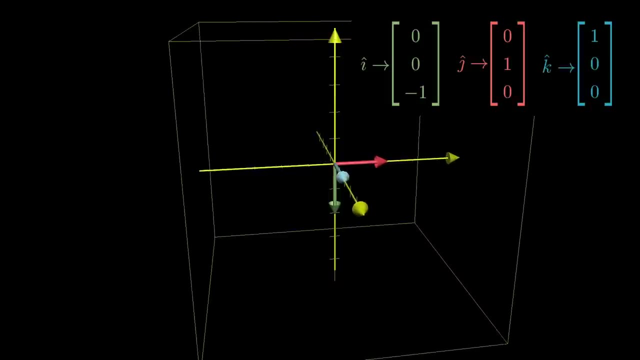 and then k-hat moves over to the x-axis at, Those three sets of coordinates become the columns of a matrix that describes that rotation transformation To see where a vector with coordinates lands. the reasoning is almost identical to what it was for 2x3.. 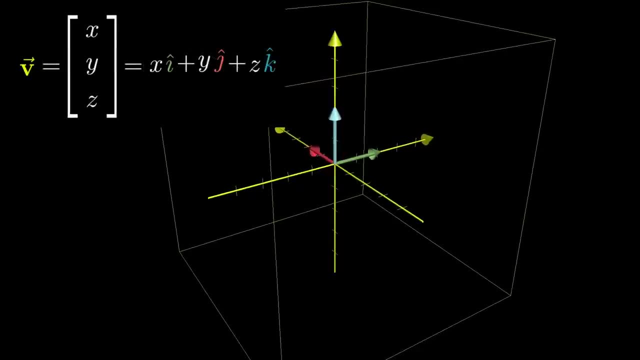 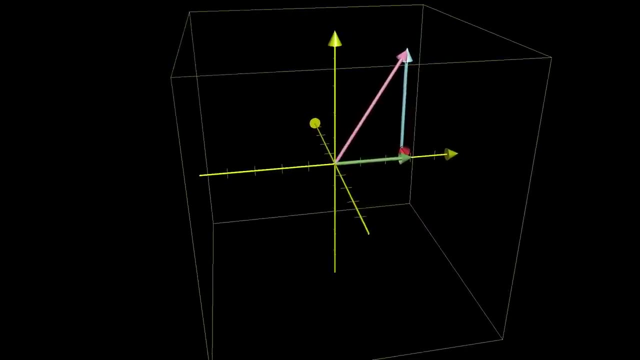 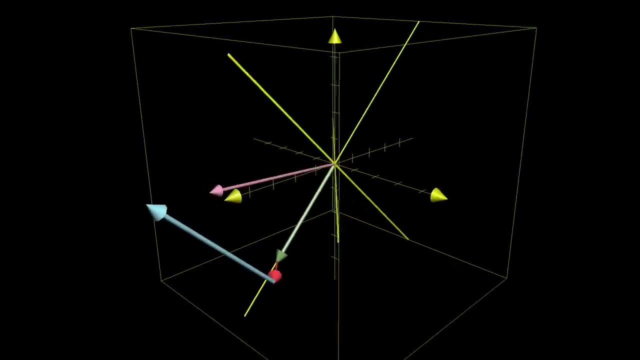 Each of those coordinates can be thought of as instructions for how to scale each basis vector so that they add together to get your vector. And the important part, just like the 2D case, is that this scaling and adding process works both before and after the transformation. 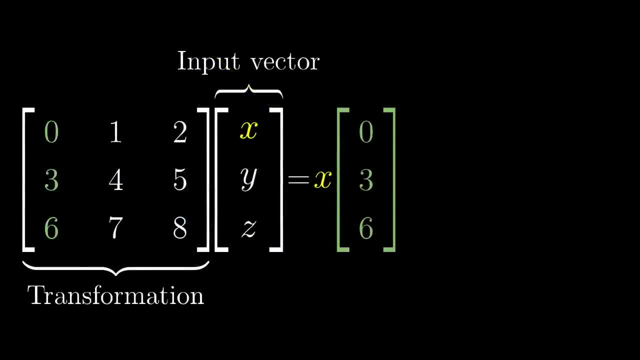 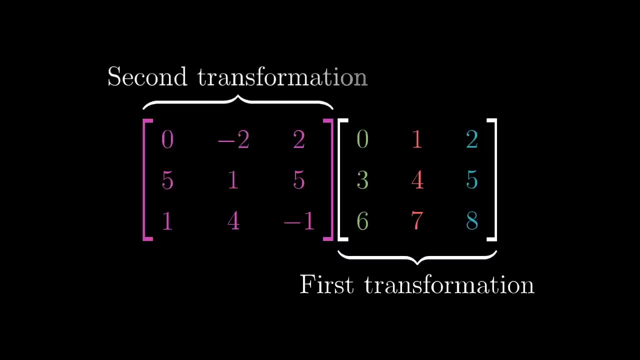 So to see where your vector lands, you multiply those coordinates by the corresponding columns of the matrix and then you add together the three results. Multiplying two matrices is also similar. Whenever you see two 3x3 matrices getting multiplied together, you should imagine first applying the transformation encoded by the. 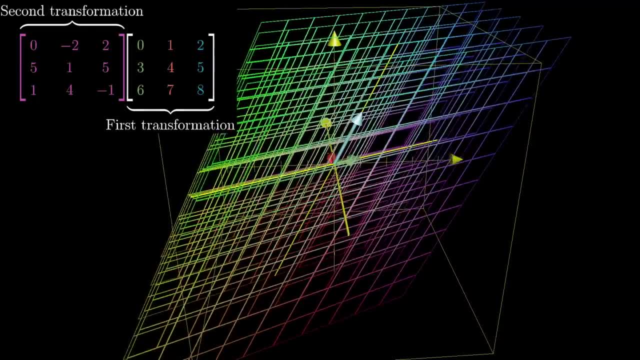 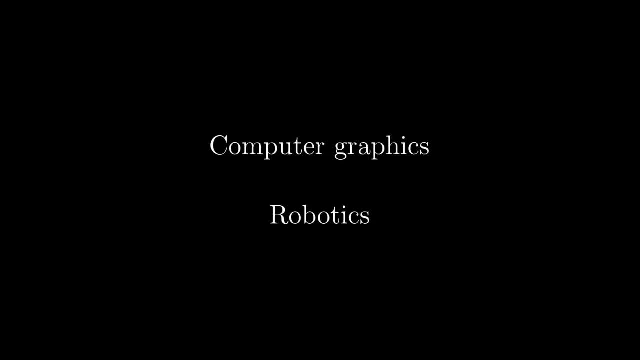 right one, then applying the transformation encoded by the left one, It turns out that 3D matrix multiplication is actually pretty important for fields like computer graphics and robotics, since things like rotations in three dimensions can be pretty hard to describe, but they're easier to wrap your mind around. 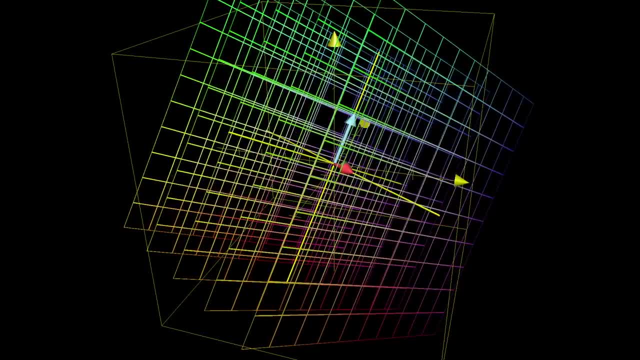 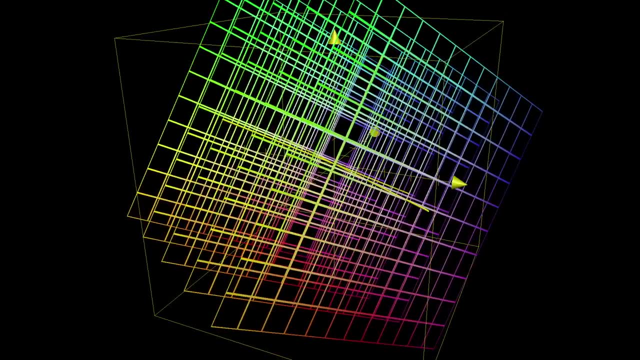 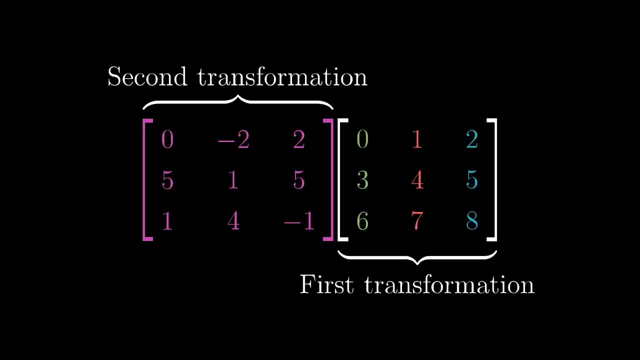 Subtitles by the Amaraorg community round, if you can break them down as the composition of separate, easier-to-think-about rotations, Performing this matrix multiplication numerically is once again pretty similar to the two-dimensional case. In fact, a good way to test your understanding of the last video would be to try to reason. 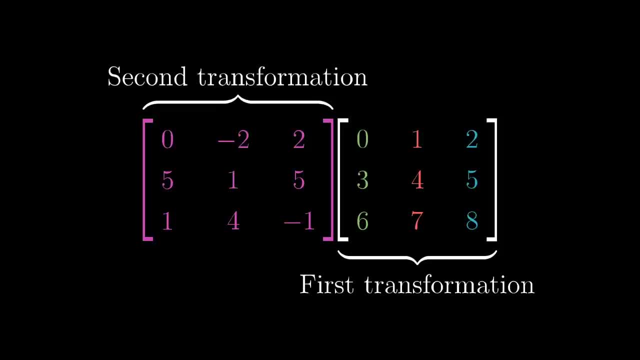 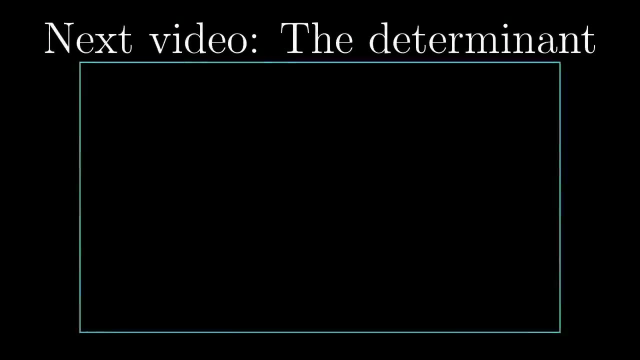 through what specifically this matrix multiplication should look like, thinking closely about how it relates to the idea of applying two successive transformations in space. In the next video I'll start getting into the determinant.